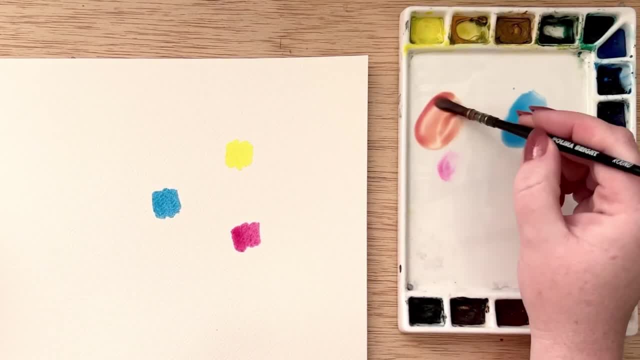 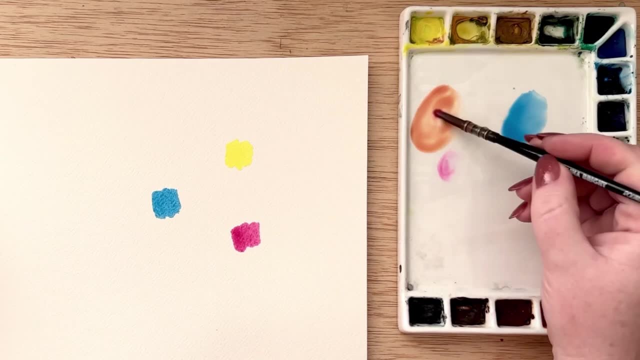 So now to create the secondary colors in our color wheel, we are mixing two primary colors together. We're going to be using a yellow, magenta and cyan color theory, which produces an even mixture. So here I'm mixing yellow and magenta together to make sure that both colors 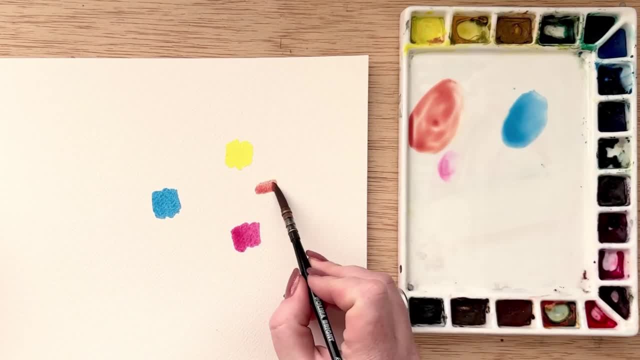 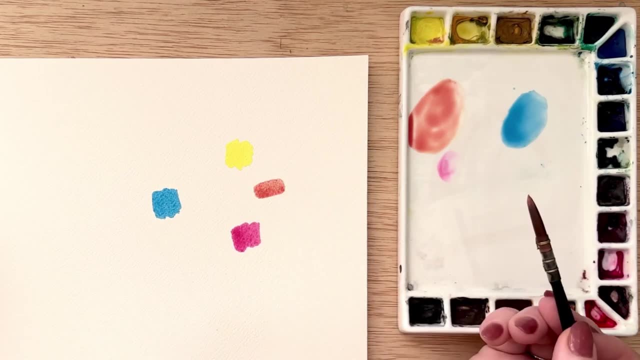 are represented evenly. It's not leaning yellow and it's not leaning magenta, And you'll see we've actually created red. So that's the interesting thing about this color theory is, using yellow and magenta, secondary color becomes red. The reason I like to paint the secondary color first. 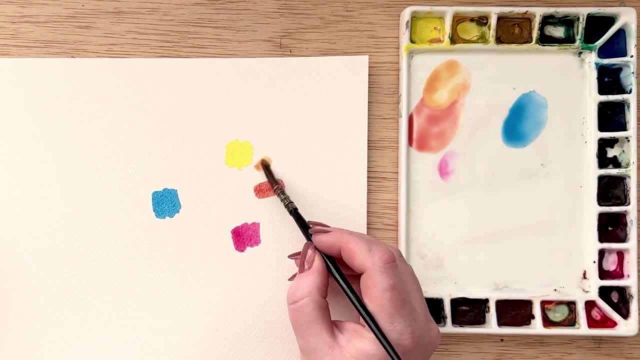 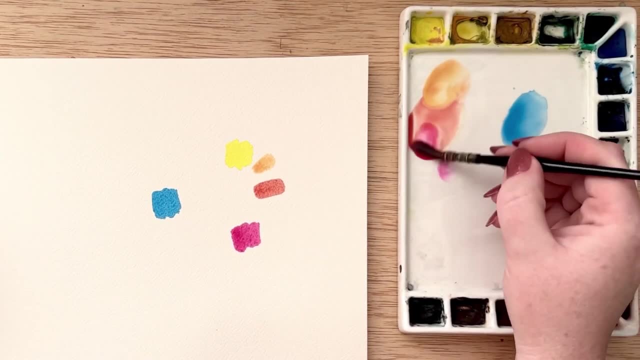 is because now I can just add a little bit of yellow to that mixture we already have And we get our first tertiary color, So it's obviously leaning more yellow. Then I add a little bit of magenta to the mixture we already have And now it's leaning more magenta without. 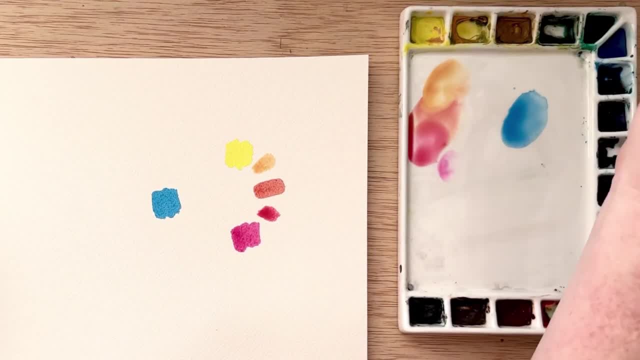 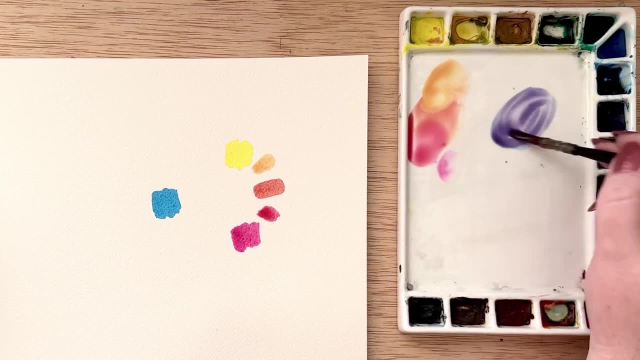 being pure magenta. So that's how we can get those mixtures that are in between the secondary and the primary colors and they're called tertiary colors. So now we're going to mix up the secondary color between magenta and cyan, and that is purple. 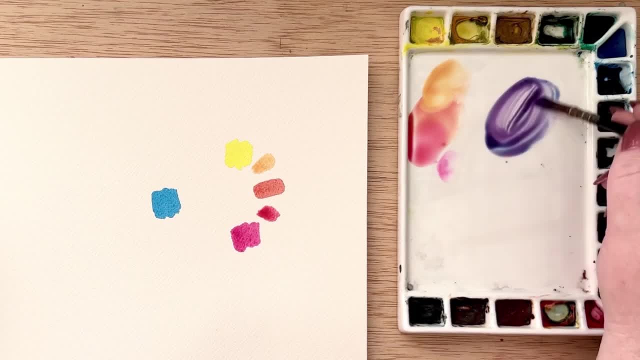 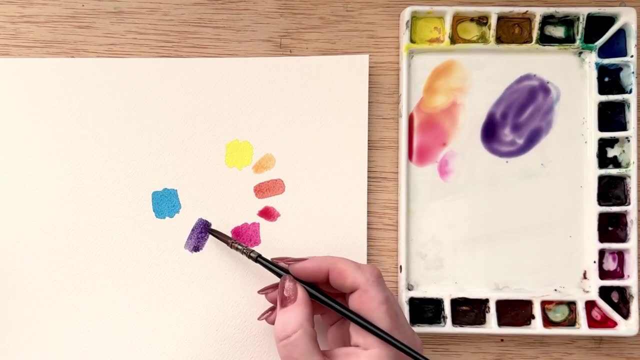 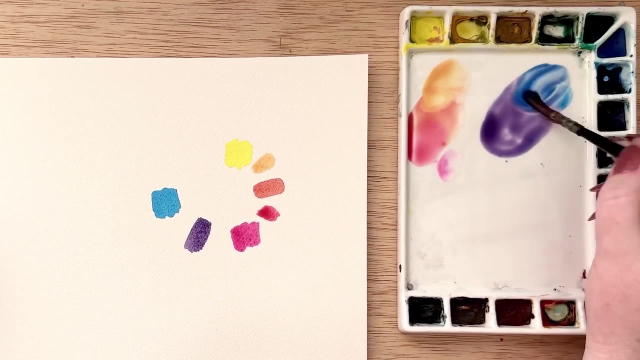 So, again, I'm just making sure that this purple is not leaning blue and is not leaning magenta, So I just go back and forth between adding the paint until I feel like it's an even mixture. Now, one of the things that helps me to know in this case that it's an even mixture is when you 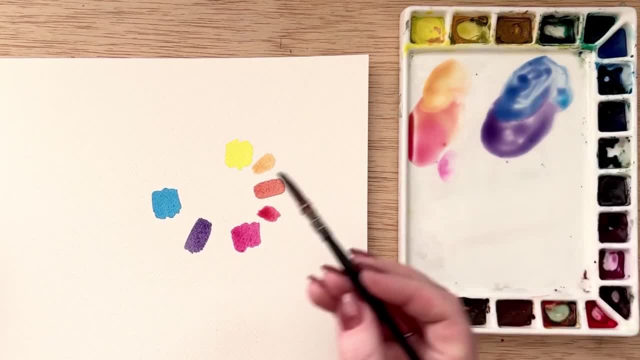 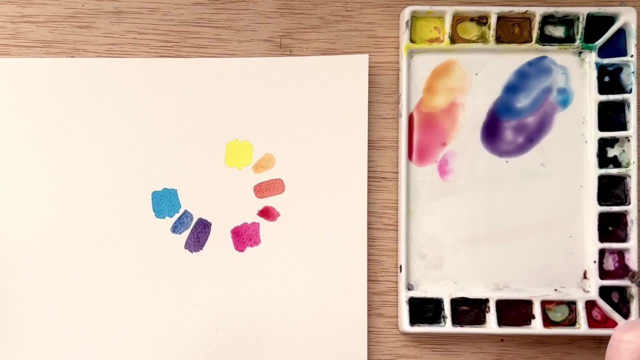 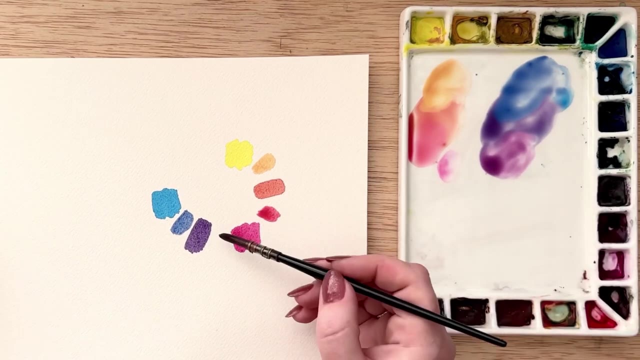 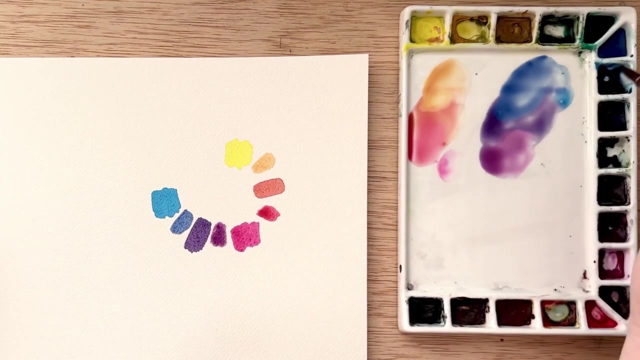 add more cyan to purple, you actually get the color blue. So blue ends up becoming a tertiary color, which is kind of cool. So cyan and purple makes blue. And then you add more magenta to that mixture we already had and you get what they call magenta purple. So it's just a really pretty. 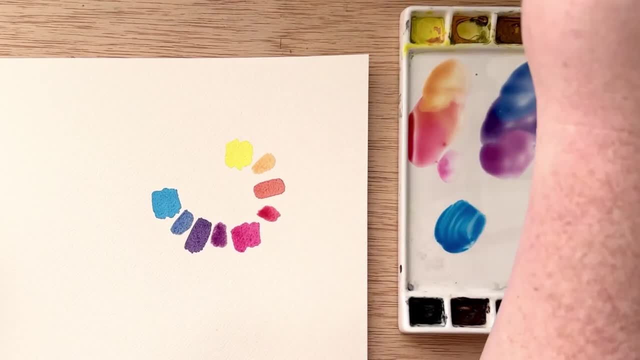 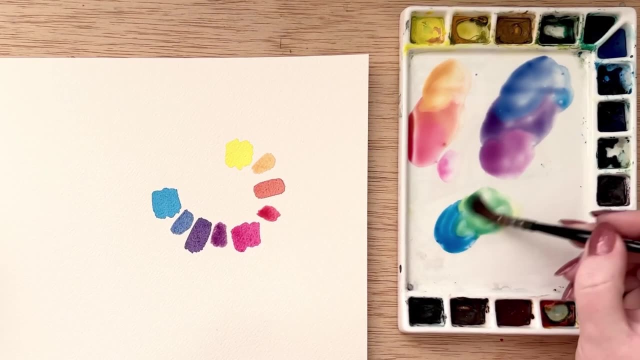 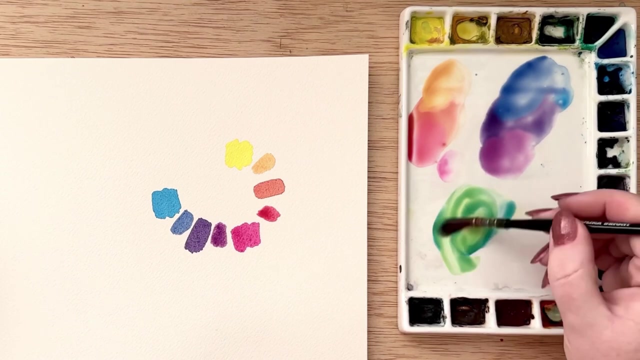 bright purple color. I love that color. Now we're going to mix cyan with yellow to get, as you guessed, green, And it's a very beautiful bright green And I wouldn't focus too much on that. I just want to make sure that your mixtures are exactly 50-50- equal, because there's just no. 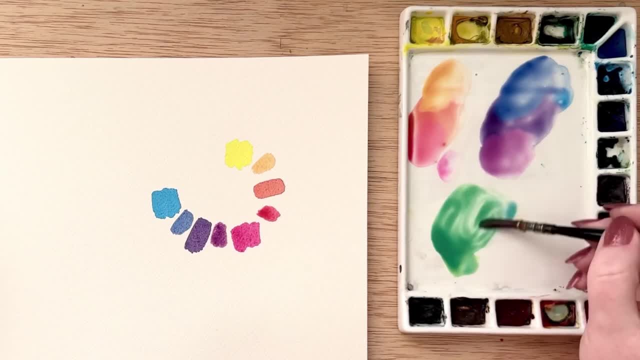 way to measure that. The only way you'll be able to tell if something is equal is just by how it looks to you, And because you're human, there's going to be error in that in some way. Because now, looking back at this, I'm thinking that that green leans a lot more cyan than I would have. 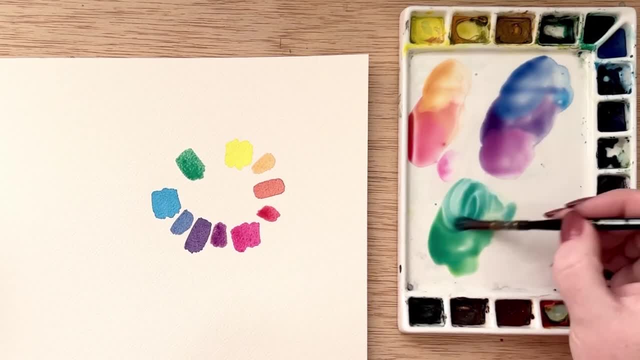 liked. So that's on me. I should have added more yellow. That's okay, I'm human. But then I add a little bit more cyan to this mixture And then I add a little bit more magenta to this mixture And 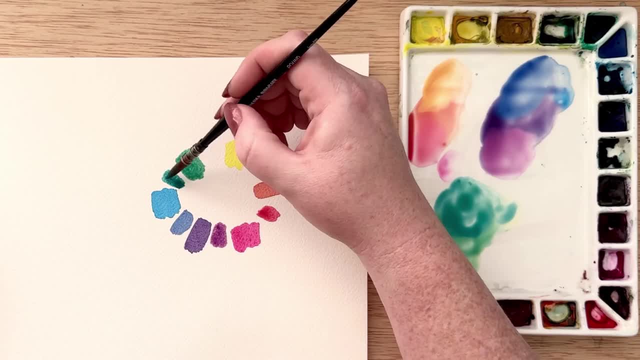 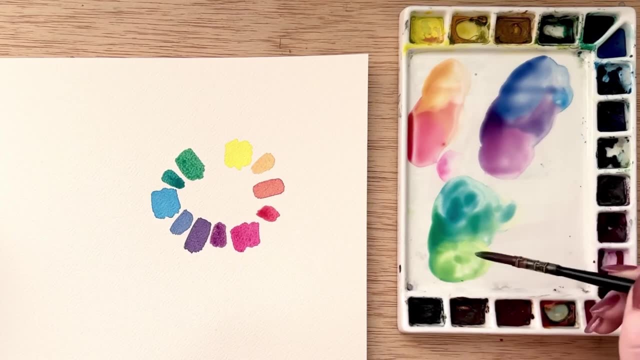 then I add a little bit more magenta to this mixture And then I add a little bit more cyan to this mixture And I get a beautiful blue-green between those two. And then I'm going to add a little bit of yellow to that existing mixture and get that beautiful yellow-green chartreuse color. That is one of my. 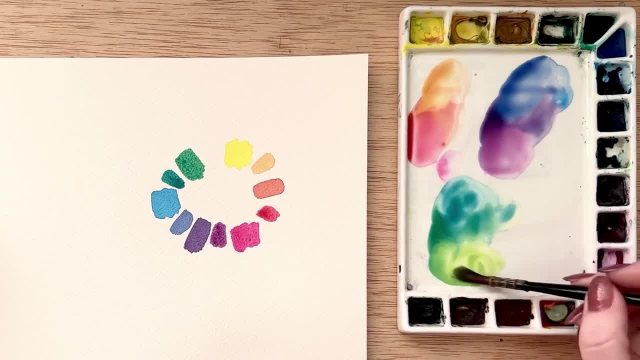 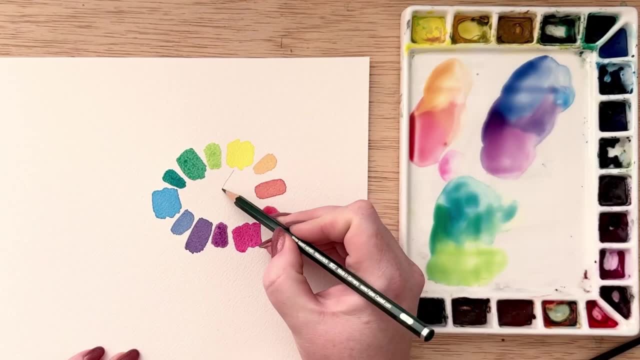 absolute favorite colors. It is so punchy and bright And with the completion of this color, we have all 12 of our colors. So the primary colors, secondary and tertiary colors represented. Now we're going to talk about complementary colors. Complementary colors are opposite of. 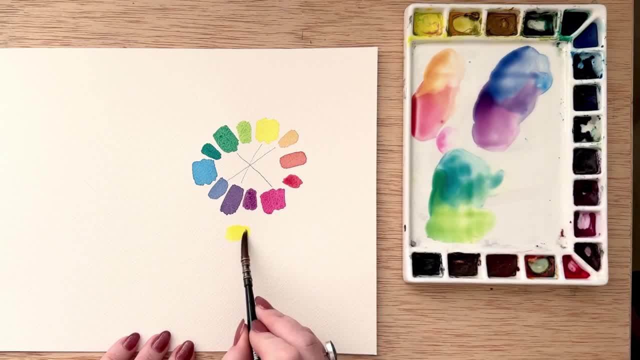 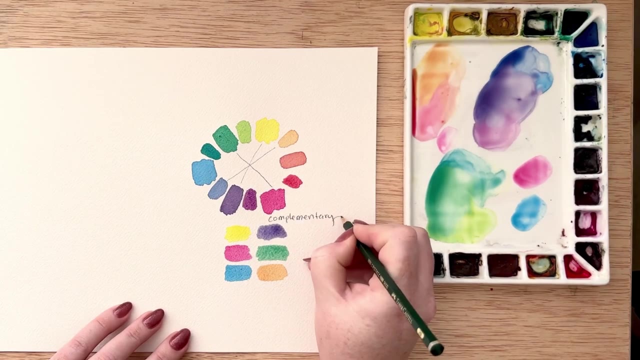 each other on the color wheel. So an example of this would be green and magenta, purple and yellow and blue and orange. Now you might ask yourself, why does it even matter that? I know what complementary colors are. Well, complementary colors actually mute each other. So if you mix an even ratio of complementary colors, 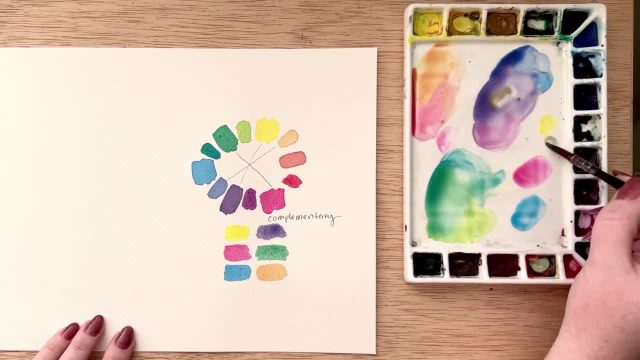 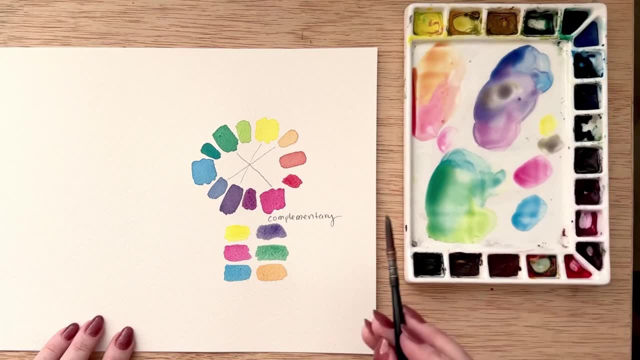 together, like here I'm doing, yellow and purple- you actually cancel the colors out, So the color becomes gray, And this works with every color in the color wheel. So I'm going to do a little bit of a color that is opposite of each other on the color wheel. You will cancel the colors out and get a. 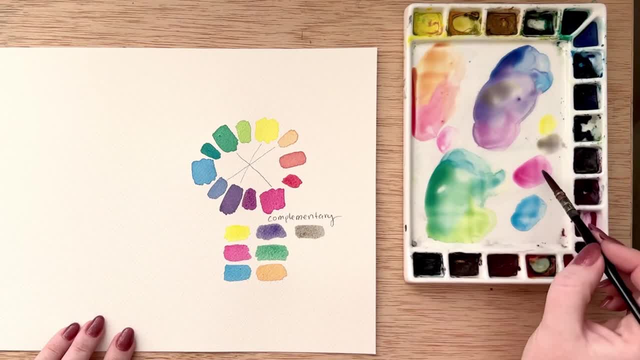 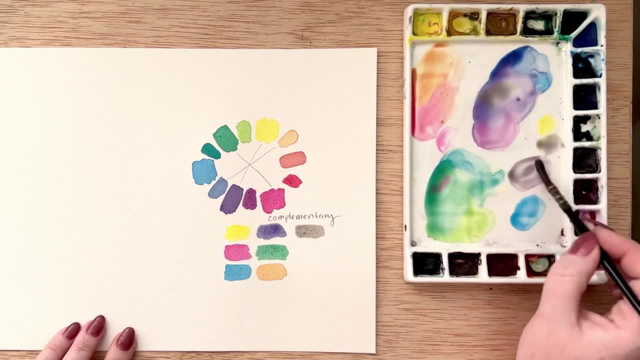 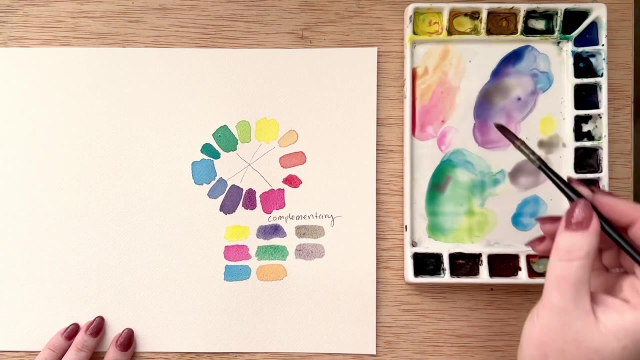 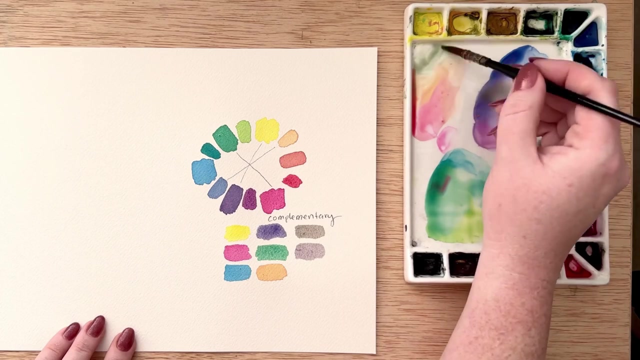 gray, dull color for each one. It's also important to know that complementary colors enhance each other, So when they're next to each other in a painting, they increase the contrast and the interest in the painting just by being together. medium shoot. 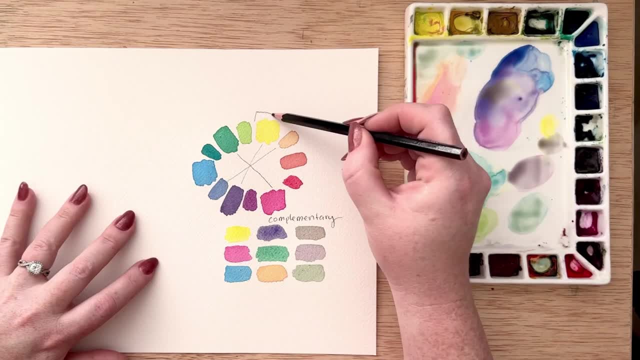 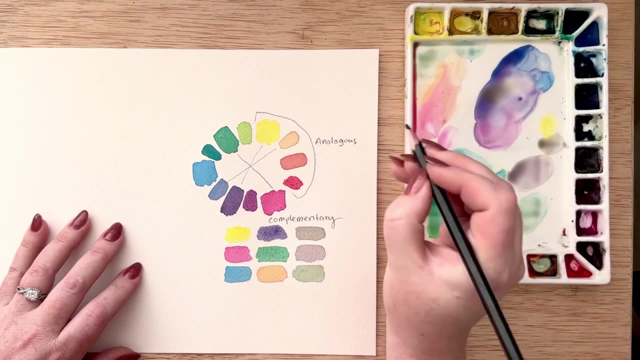 The next type of grouping is called analogous colors, and it is three or more colors that are next to each other on the color wheel, And these colors enhance each other. they act as accents and contrast. The next color grouping we're going to be talking about is triadic colors. triadic colors. 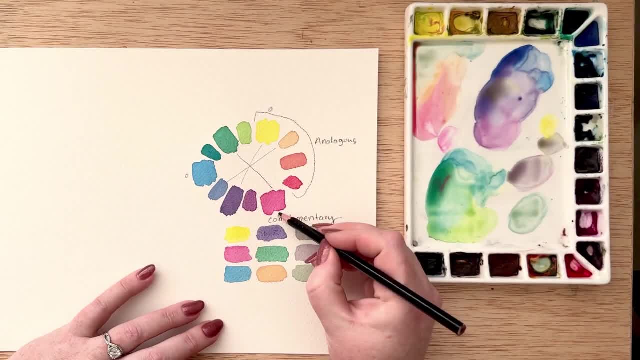 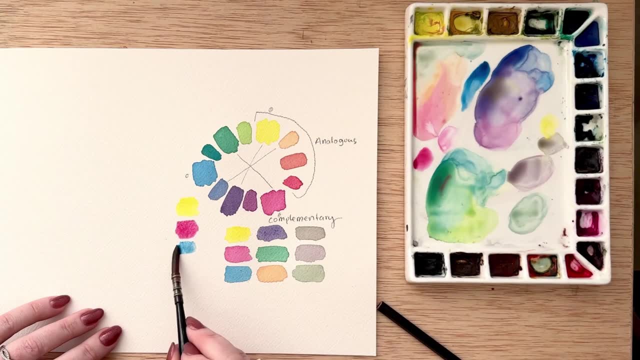 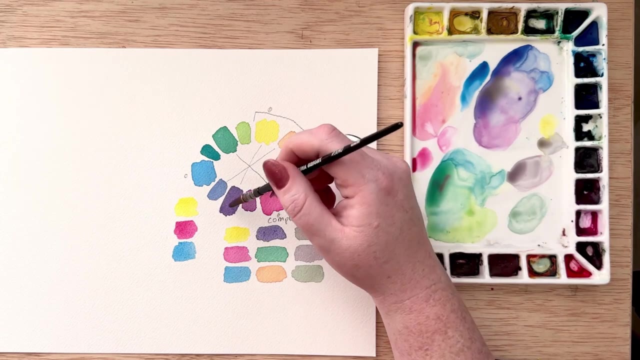 we're going to be talking about is 회. Colors are three colors that are evenly spaced on the color wheel, making the points of a triangle. So, like we talked about in the beginning, the primary colors of cyan, magenta and yellow create a triadic grouping. 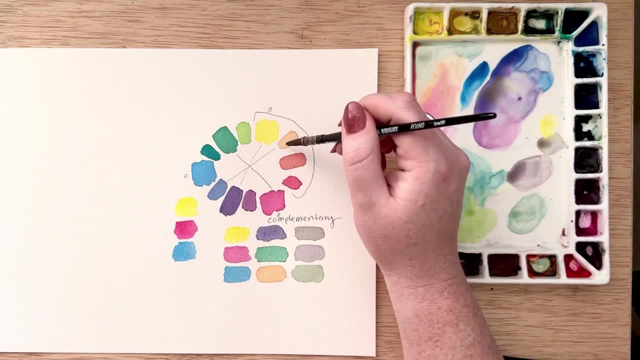 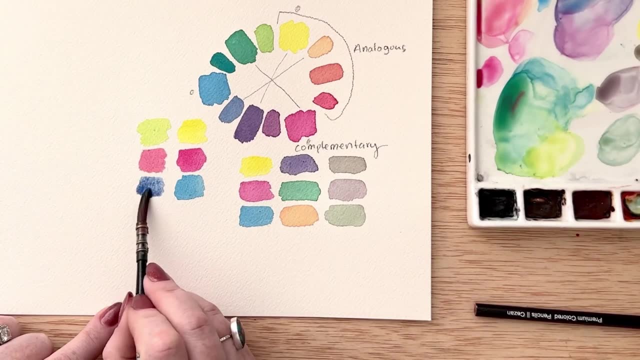 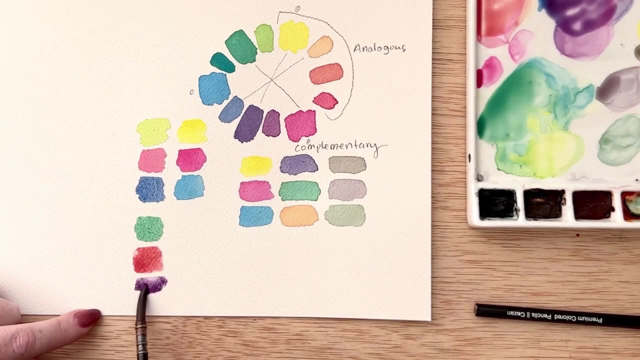 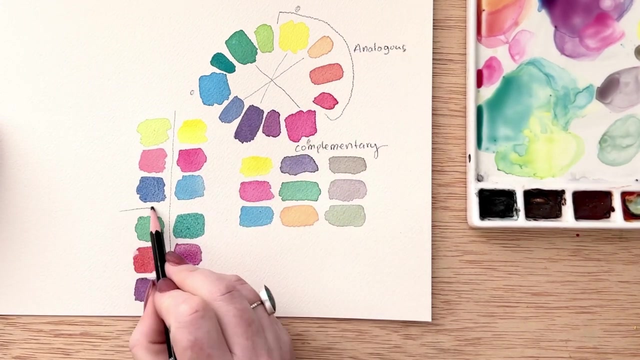 There's also three other triadic groupings. There is the bright yellow-green with the red, magenta and blue. Then there is green, red and purple. Purple, blue-green, magenta-purple and orange. Triadic colors are just another way to create a harmonious color palette that adds a lot of contrast with accent colors. 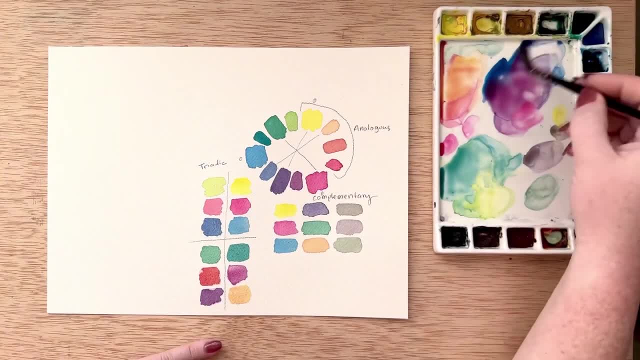 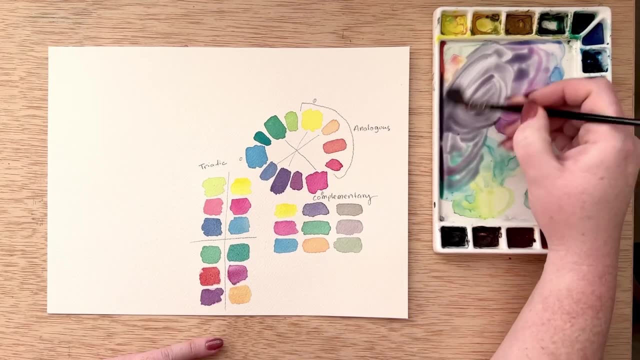 And how do you make black? Well, you take all of the colors on the color wheel and you mix them together to get black. So really, if you want to mix black in a more simple way, cyan, magenta and yellow will get black. 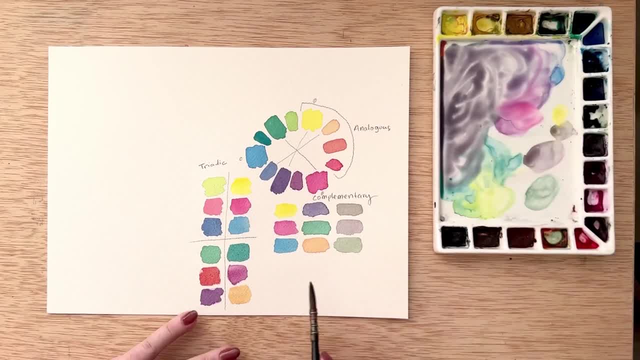 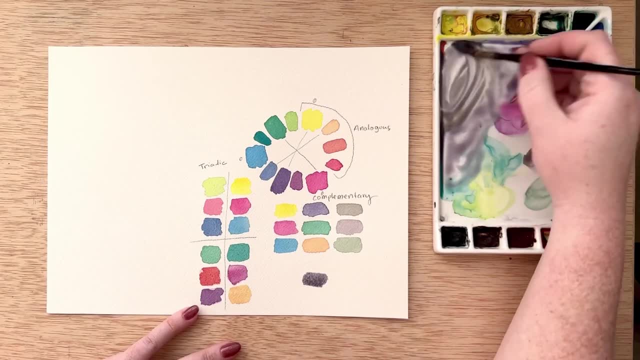 Now, as I'm mixing all of this, and I even put it on the paper, I feel like it is leaning purple. So how do I fix that? I add yellow, because yellow cancels out purple, which goes back to our complementary colors. 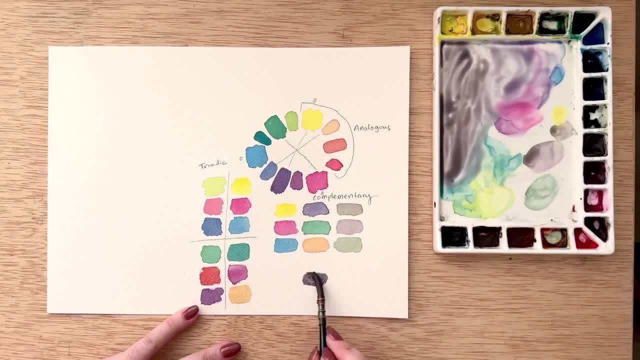 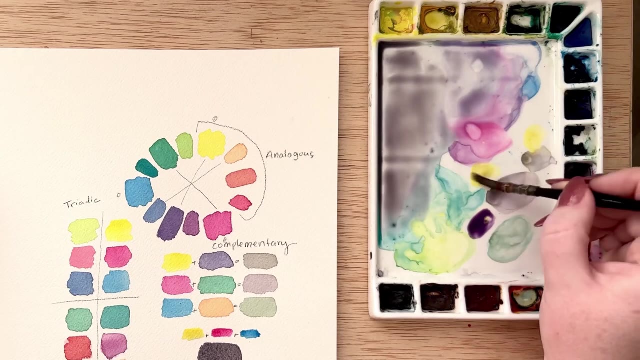 And you can see how much more black that gets. Beautiful Color theory working right in front of our eyes. So, just as a reminder, yellow, Cyan and magenta make black And as I was painting this, I remembered something I wanted to tell you about complementary colors. 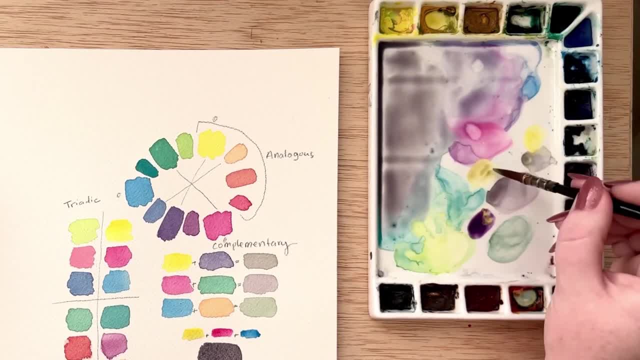 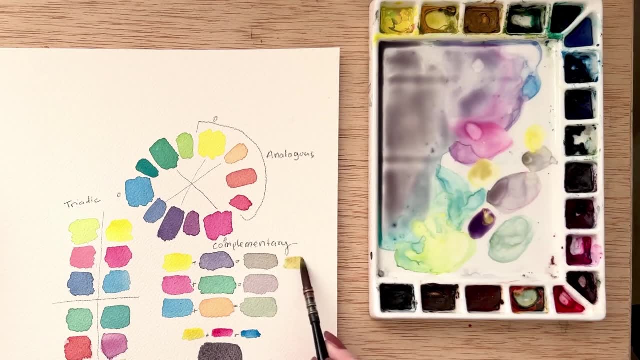 If you add the tiniest bit of a color's complement, like I'm adding purple to yellow in the tiniest bit- it doesn't neutralize yellow, but it darkens it enough to become a shadow. So this is how you make shadow colors for your paintings. 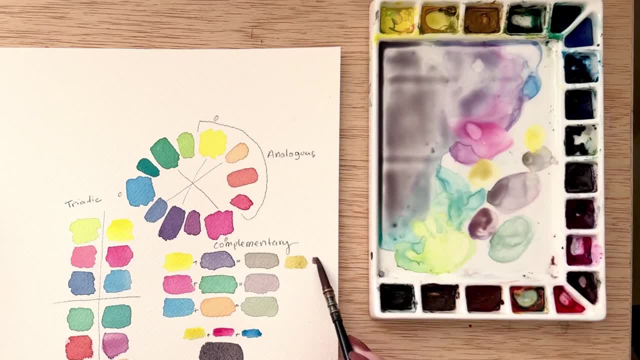 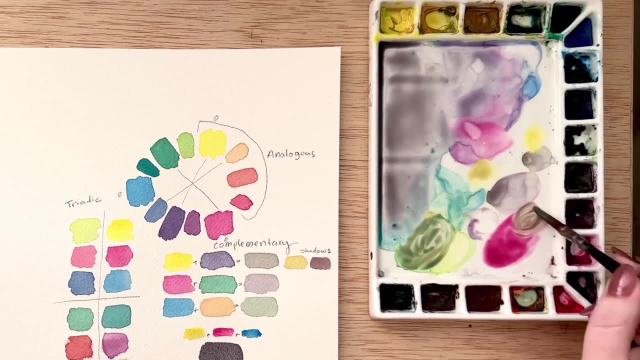 Is you just add the tiniest bit of a color's complement and you get the black And you get a perfect darker hue that looks very pleasing to the eye when you want to make shadows on any object that you want to paint. 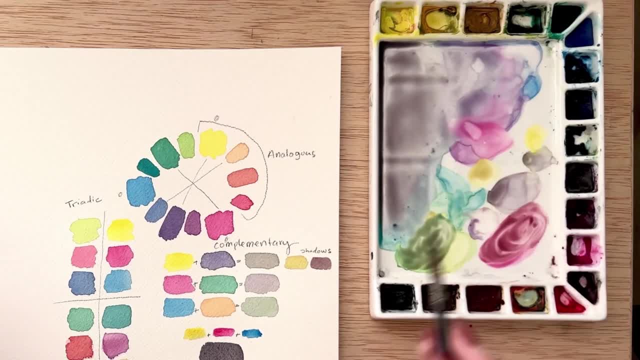 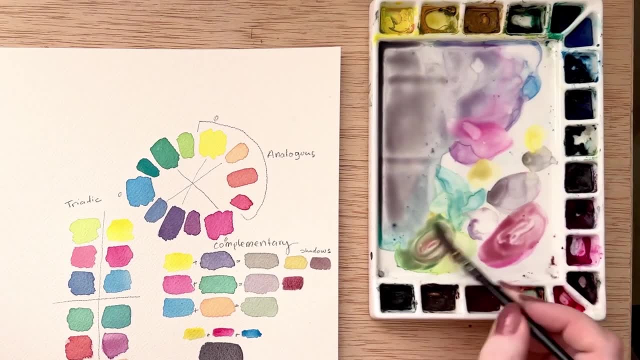 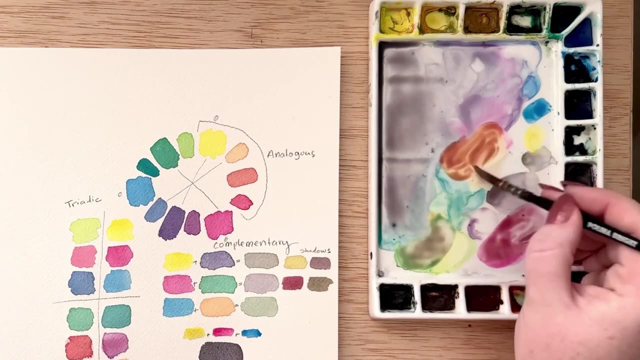 So same here for the magenta with the green. Adding a little bit of green to the magenta makes such a pretty darker rose color, And vice versa. adding magenta to the green makes a beautiful green color, And I use this technique a lot in my floral paintings to get a deeper rose color. 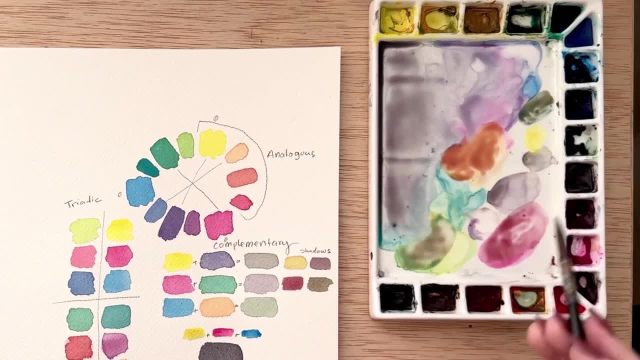 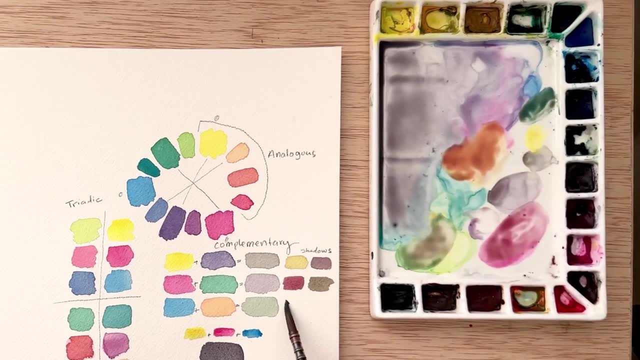 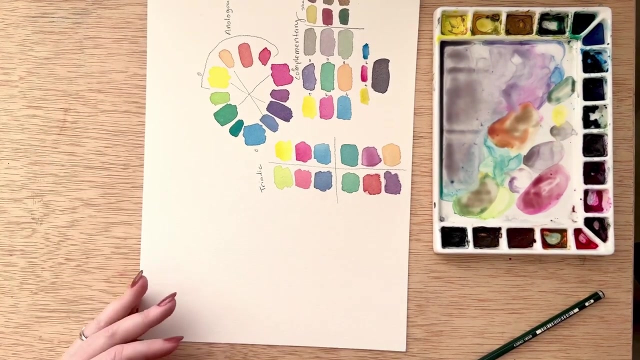 and a deeper, more natural-looking green color. Now I'm going to turn my paper and we're going to do an exercise in blending, So I'm getting rid of some of that black on my palette. So I'm getting rid of some of that black on my palette. 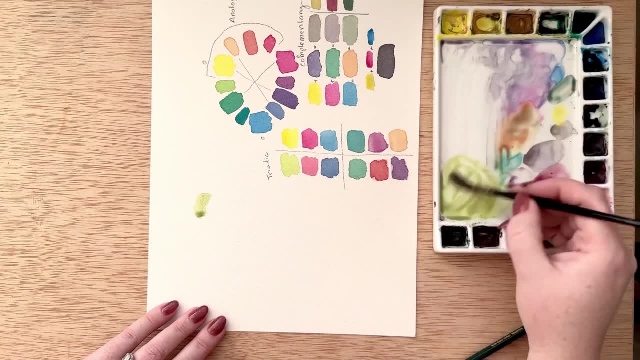 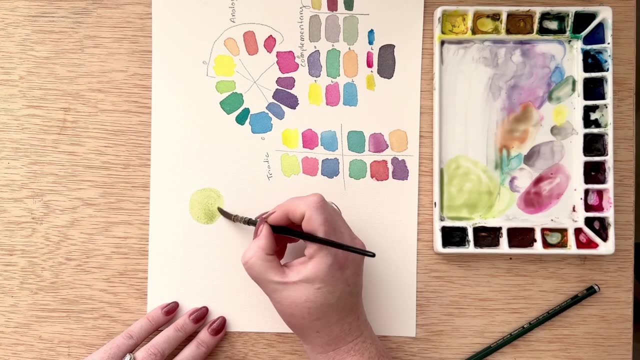 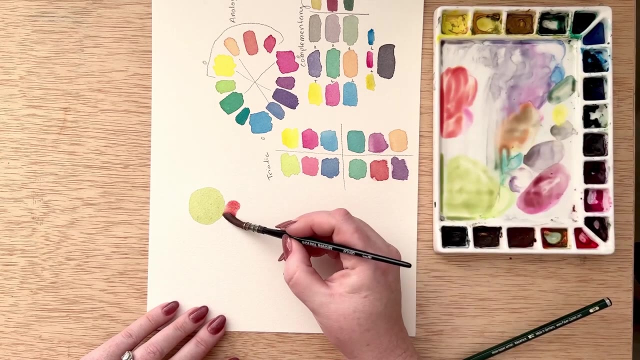 So I'm getting rid of some of that black on my palette and I'm starting with the bright yellow-green And I'm taking inspiration from what I have on my color wheel and my charting here. So I'm doing the bright yellow-green which made me want to do the triadic colors in that lower left group. you can see right there. 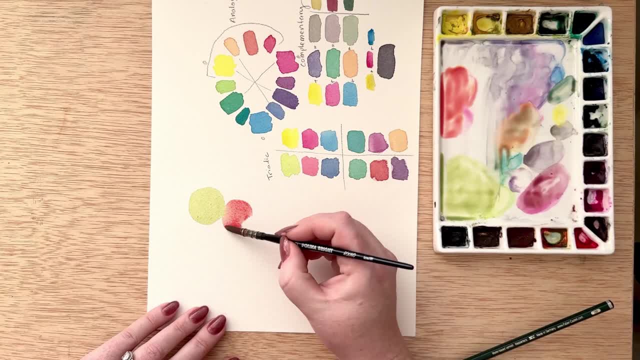 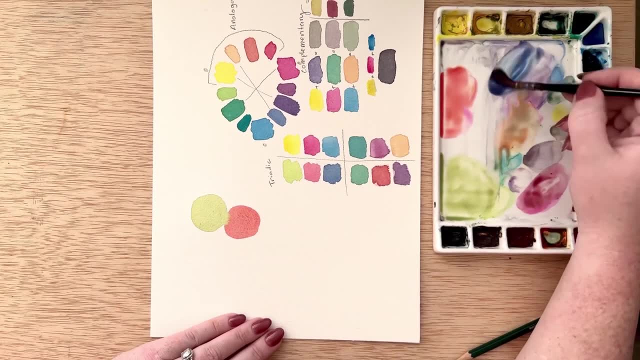 The next color is that- magenta-red. So then I did magenta-red next to that, and it's just amazing how beautiful those colors are together that I probably never would have put next to each other. And then the next color is blue. 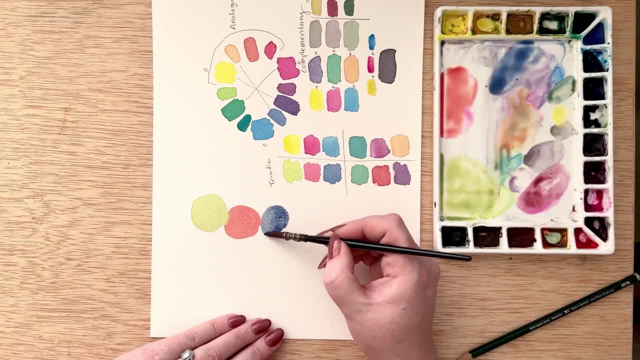 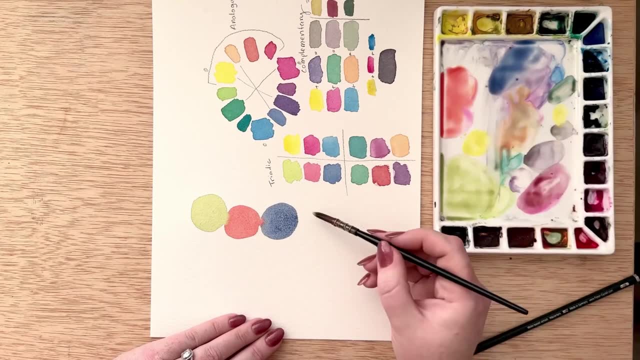 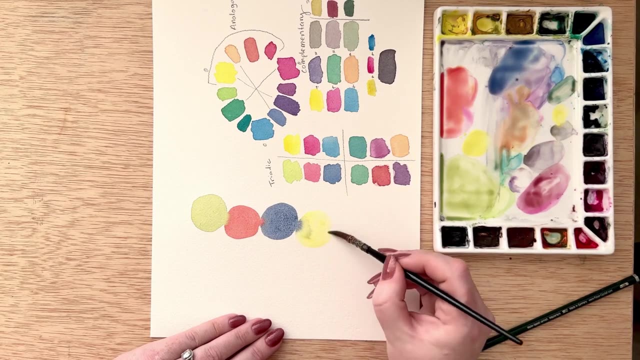 And those three colors together and watching them blend is just a really fun exercise. And then I just started adding more colors from my palette to get continuous blending technique. So with this technique you just want to make sure that you have enough water to pigment on your brush. 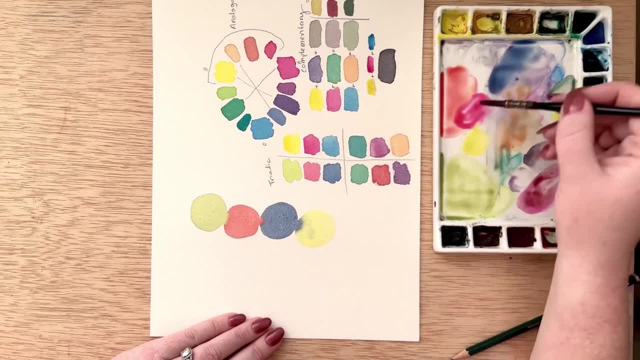 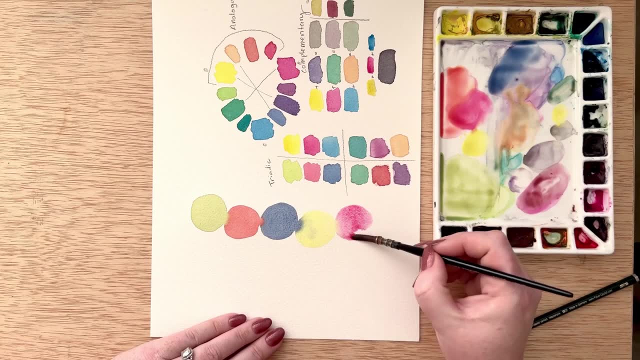 that it's runny enough that everything blends. If it's too dry, you won't get a good blend, And if it's too wet, it will blend too much. And circles are just the best for this technique. I could paint a million touching circles. 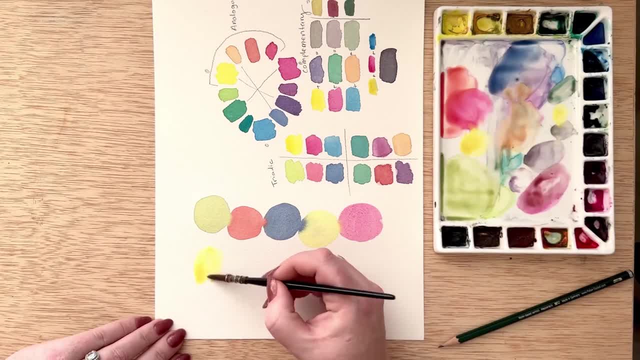 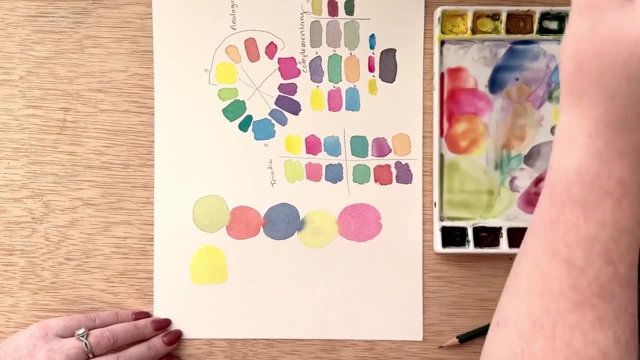 Now I'm going to make some fun shapes using an analogous pattern of color, And again that's three or more colors that are next to each other on the color wheel. So I'm sticking to the colors that I have marked off on my color wheel.